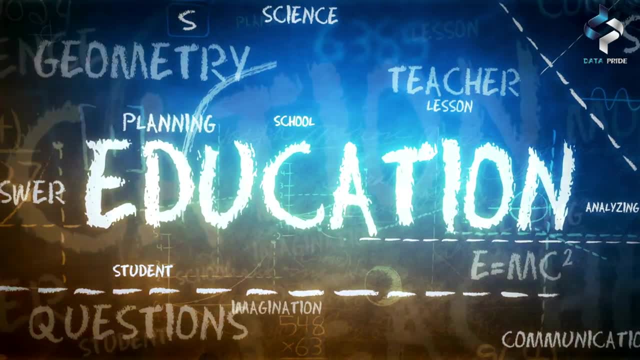 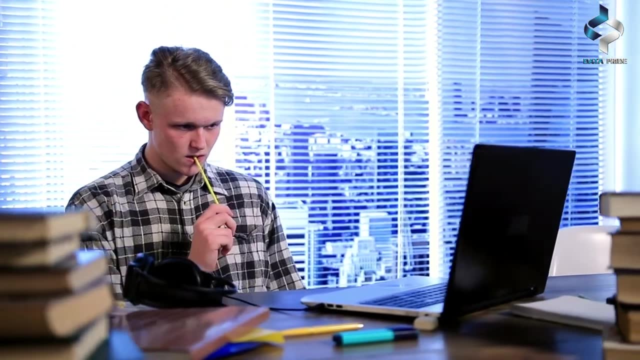 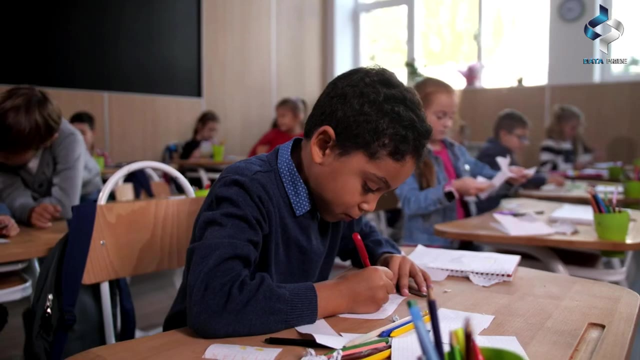 The education system is designed to identify and develop the talents of each student, providing them with the necessary skills and knowledge to succeed in life. In contrast, the United States education system places more emphasis on creativity, critical thinking and independent learning. The curriculum is more flexible. 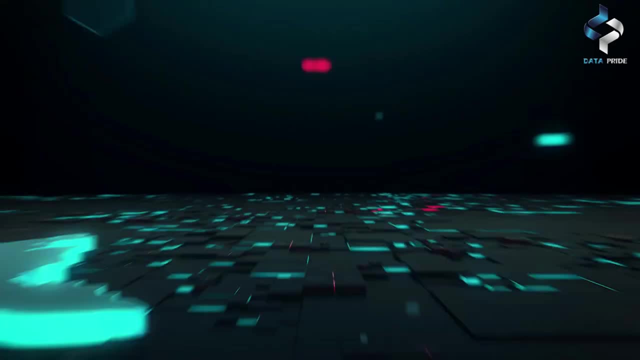 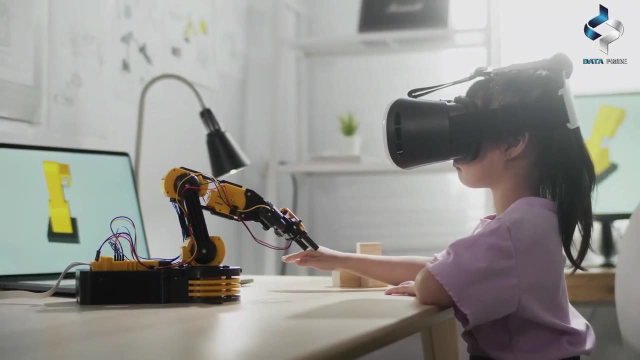 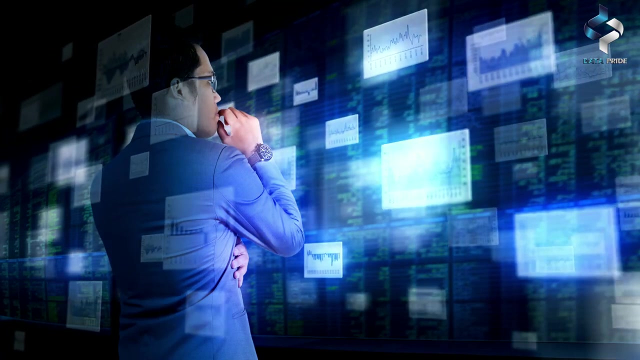 and students have more freedom to choose their courses of study. The education system is designed to develop well-rounded individuals who can think independently and contribute to society. Another difference between the education systems of the two countries is the level of investment in education. Singapore invests heavily in education, spending approximately 20% of its 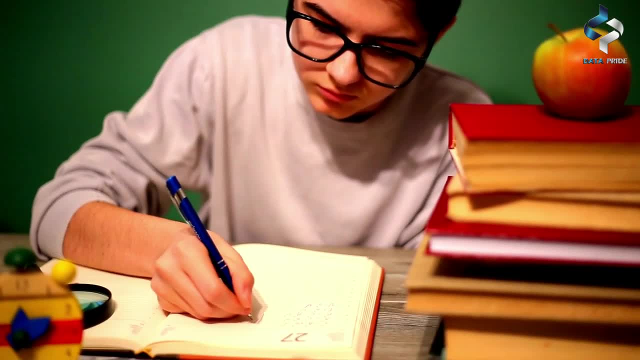 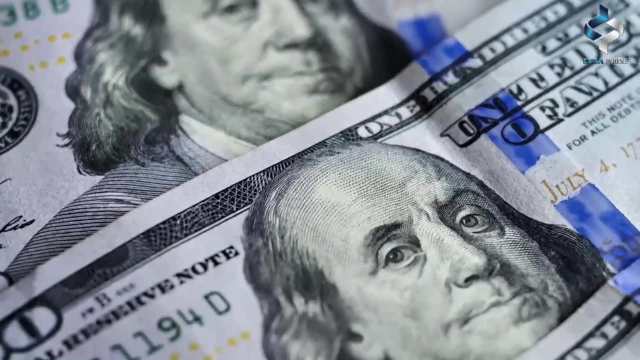 budget on education. The government provides free education for all Singaporean citizens, from primary school to university. Singapore's education system is designed to develop well-rounded individuals who can think independently and contribute to society. The United States invests less in education, spending about 6% of its budget on education. 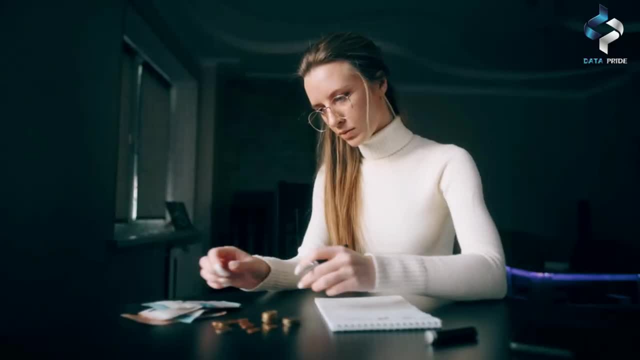 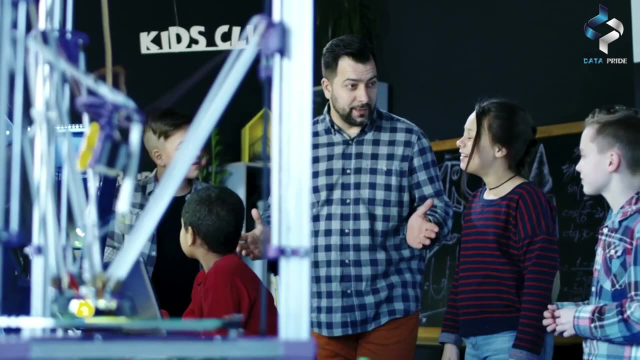 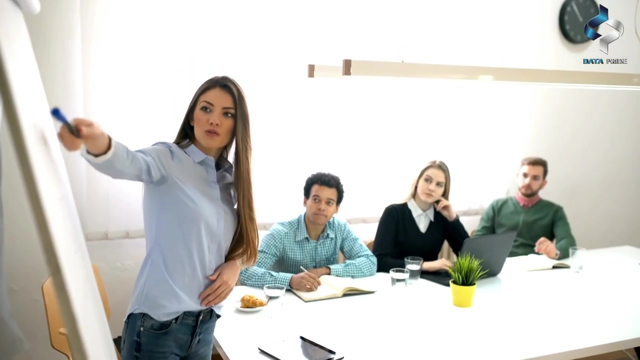 The cost of education in the United States is high, and not everyone can afford to go to college. In terms of teacher quality, both countries have highly qualified teachers. Singapore has a rigorous selection process for its teachers, and only the best candidates are selected to teach. Teachers in Singapore are also well-trained. 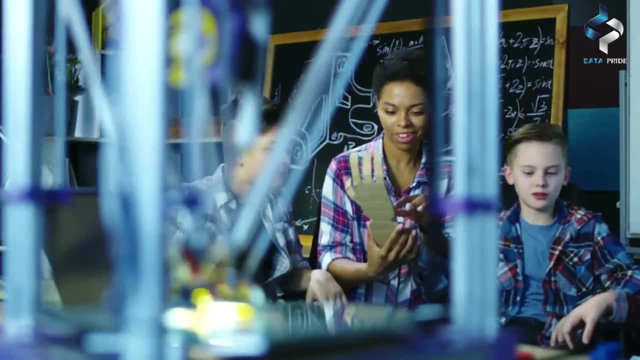 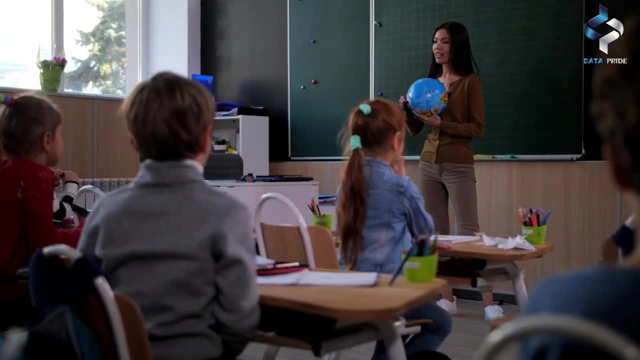 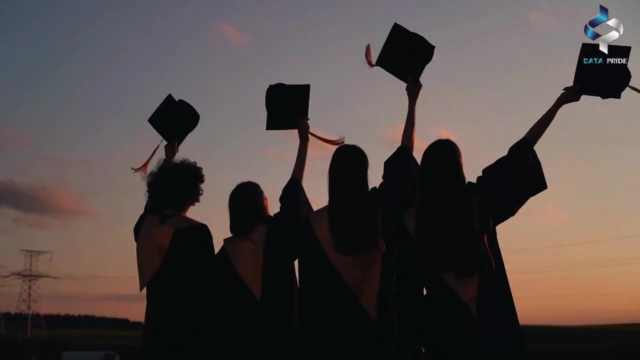 and receive ongoing professional development. In the United States, teachers are required to have a bachelor's degree and a teaching certification. However, the quality of teacher training and ongoing professional development varies depending on the state and school district. And that's a wrap on our exploration of which country has the better education system. 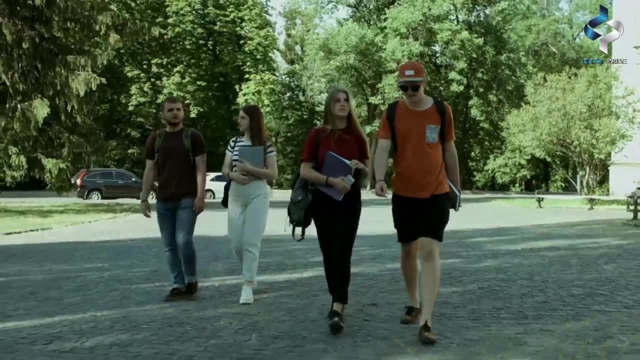 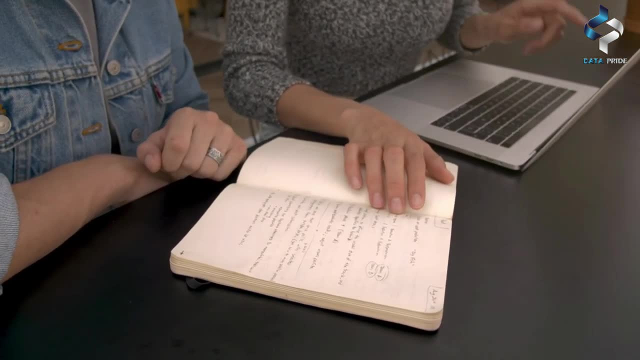 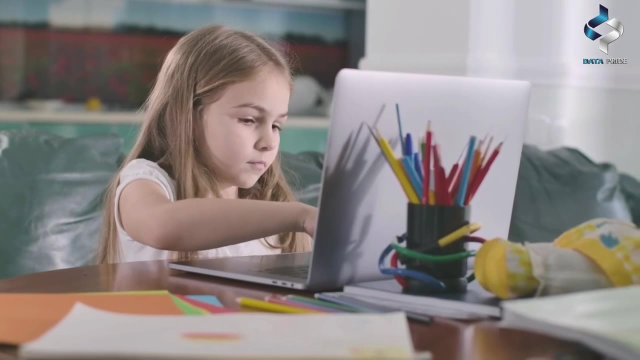 Singapore or the United States. We hope you found this video informative and insightful, and that you have a better understanding of the strengths and weaknesses of both education systems. While both countries have their unique approaches to education, it's clear that each has something valuable to offer. Ultimately, the answer to which country? 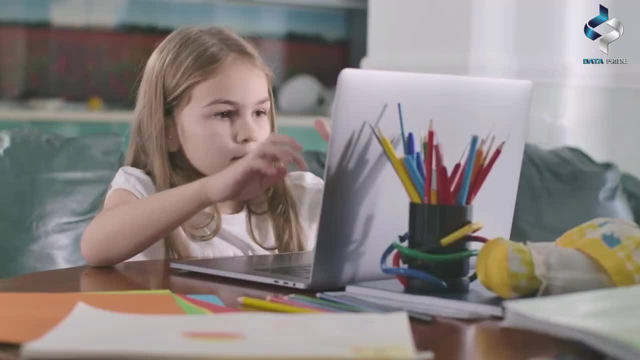 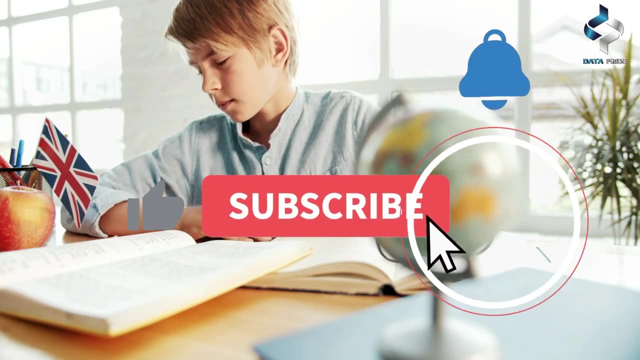 has the better education system depends on your priorities and what you value most in an education. Thank you for watching and don't forget to like and subscribe for more thought-provoking content.